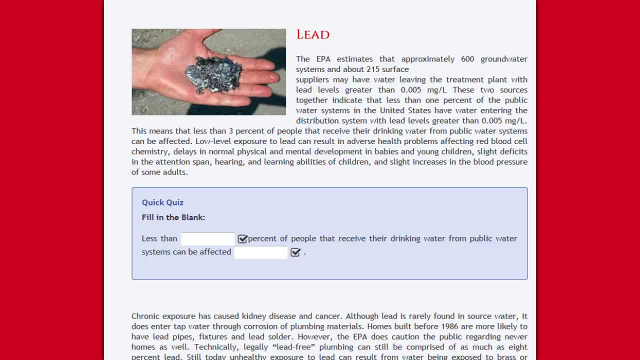 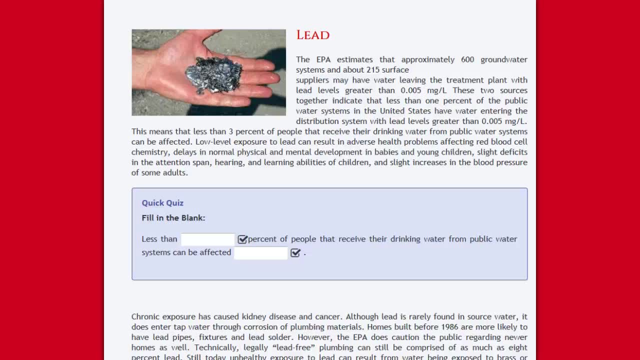 may have water leaving the treatment plant with lead levels greater than 0.005 milligrams per liter. These two sources together indicate that less than 1% water statewide supply of the greenん 我有 Nordwestgiving the distribution system with lead levels greater than 0.005 milligrams per liter. 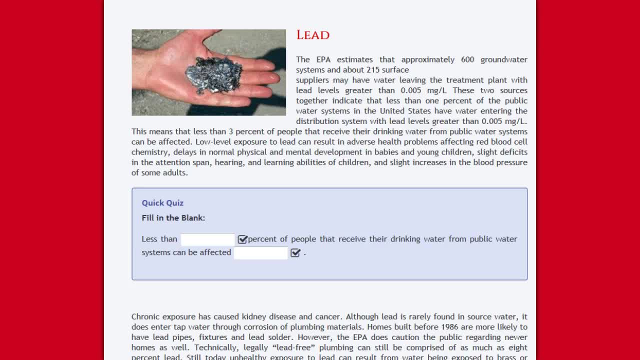 This means that less than 3% of the people that receive their drinking water from public water systems can be affected. Low-level exposure to lead can result in adverse health problems affecting red blood cell chemistry, delays in normal physical and mental development in babies and young children, slight deficits in the attention span, hearing and learning abilities. 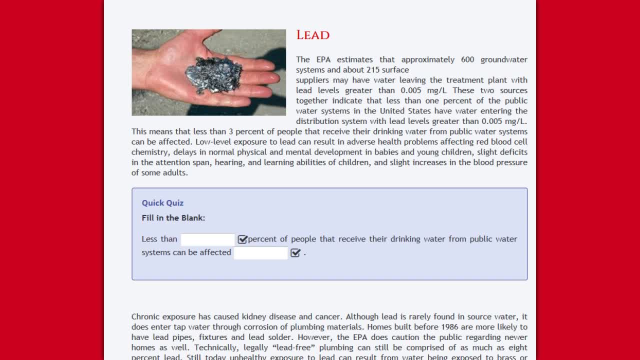 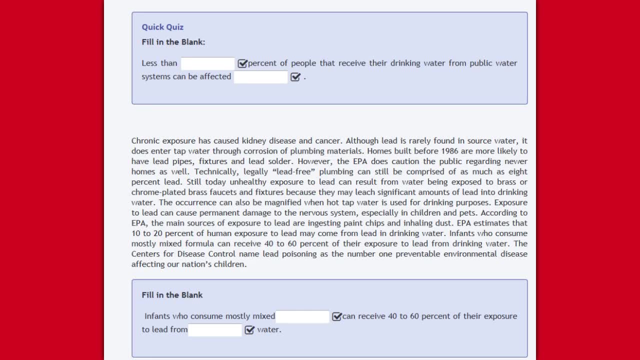 of children and slight increases in blood pressure of some adults. Chronic exposure has caused kidney disease and cancer. Although lead is rarely found in source water, it does enter tap water through corrosion of plumbing materials. Homes built before 1986 are more likely to have 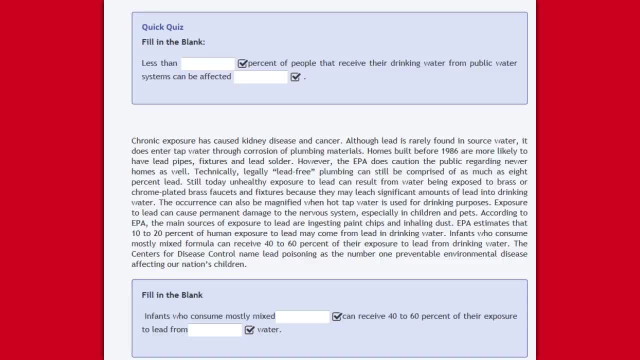 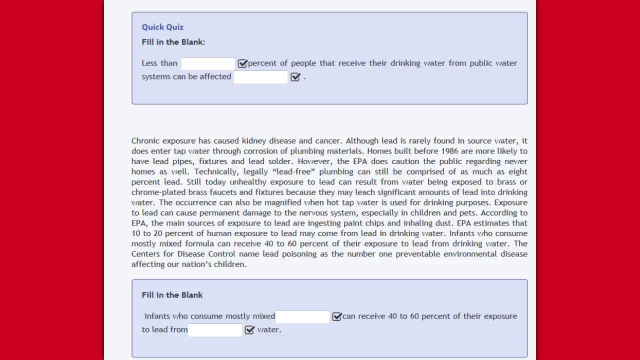 The EPA does caution the public regarding newer homes as well. Technically, legally lead-free plumbing can still be compromised of as much as 8% lead. Still today, unhealthy exposure to lead can result from water being exposed to brass or chrome-plated brass faucets and fixtures. 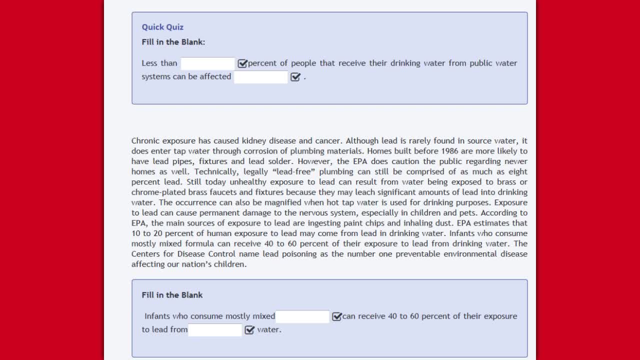 because they may leach significant amounts of lead into drinking water. The occurrence can also be magnified when hot tap water is used for drinking purposes. Exposure to lead can cause permanent damage to the nervous system, especially in children and pets. According to the EPA, the main sources of exposure to lead are ingesting paint chips. 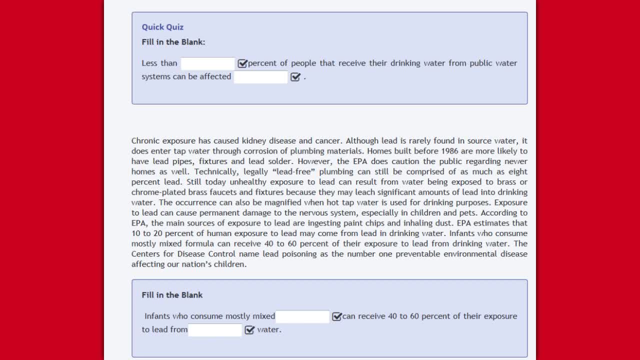 and inhaling dust. EPA estimates that 10-20% of human exposure to lead may come from lead in drinking water. Infants, who consume mostly mixed formula, can receive 40-60% of their exposure to lead from drinking water. The Centers for Disease Control name lead poisoning as the number one preventable environmental.